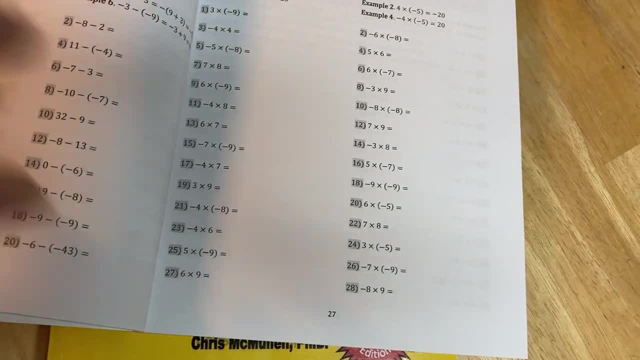 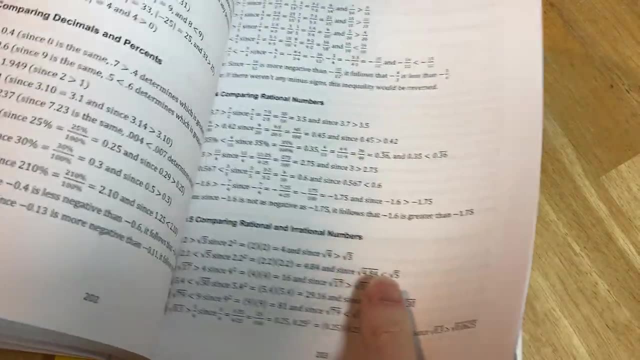 tons of problems, right, You have tons of problems. and then, when you look in the back of the book, you actually have answers to all of these problems, Which is really really good, right, You have answers to everything in the back of the book. 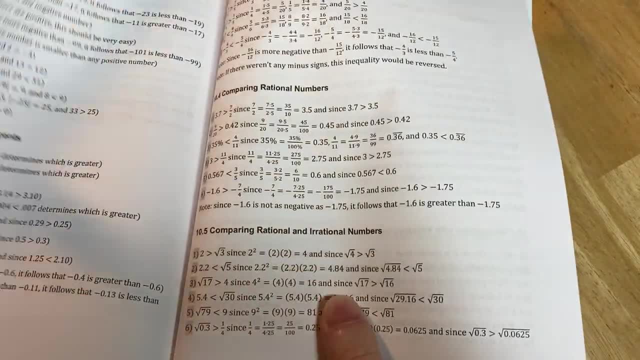 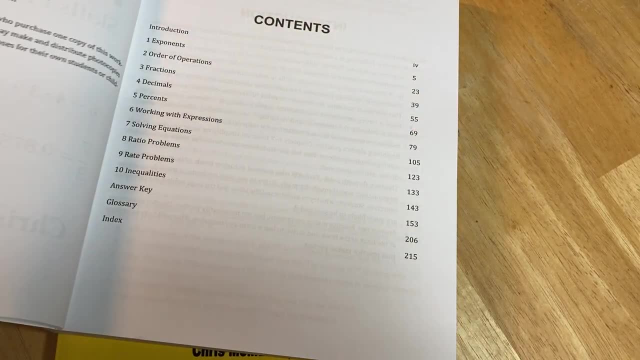 which makes it super awesome for checking your work. So let's look at some of the topics that this book covers, just to see if you think it's right for you, because, again, this is for super, super beginners. It starts with exponents. 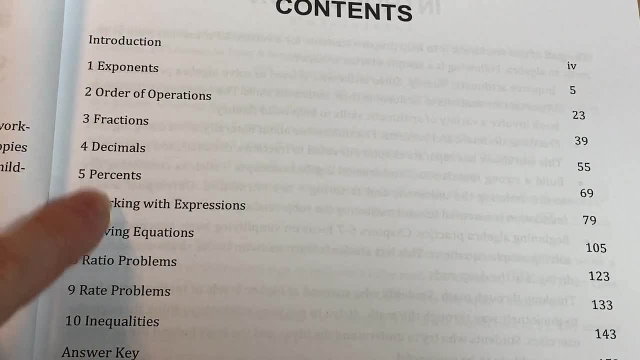 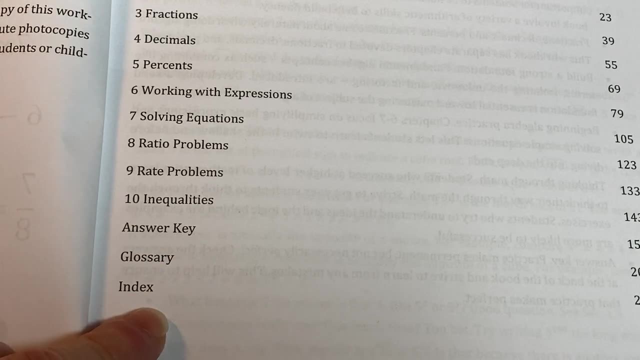 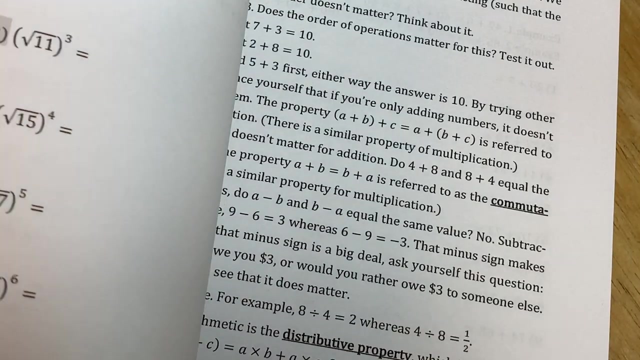 This is pre-algebra Order of operations: fractions, decimals, percents, working with expressions, solving equations, ratio problems, Rate problems and inequalities, and then you have an answer key. So this is actually where I started- mathematics I started, you know where most people start. 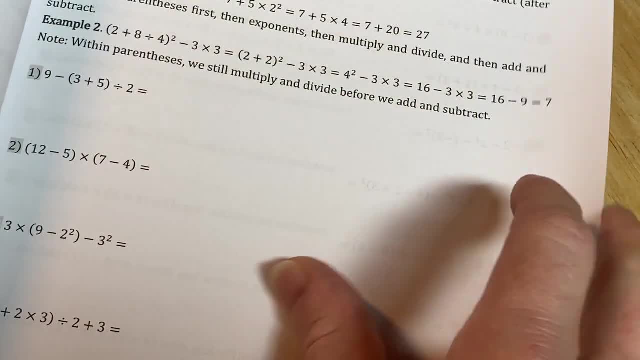 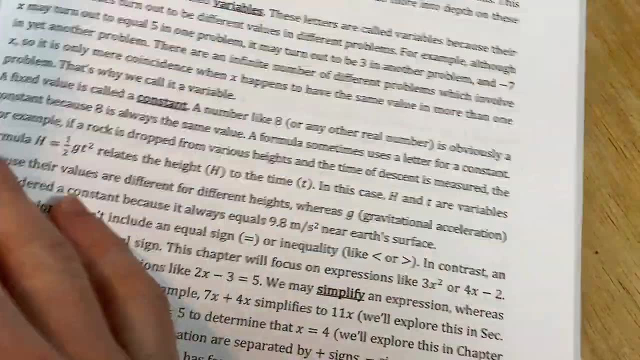 right, And it's a good place to start because you learn the basics. Now, if you feel like you know- you know about fractions, you know about decimals, you know about numbers- then you can jump ahead to this other book. And again, this is not a. 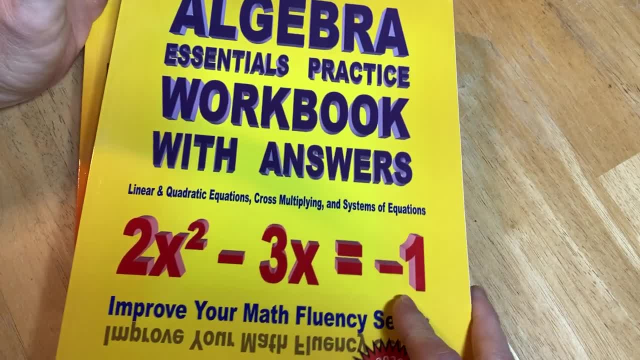 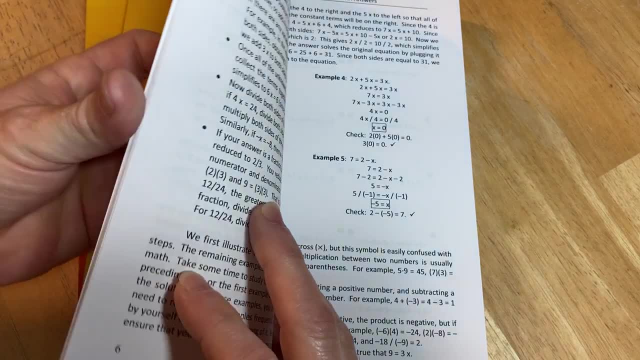 perfect book because these are workbooks. They don't have everything, but they're super affordable. And again, they have all the answers. This is Algebra Essentials Practice Workbook with Answers. This one has a little bit more advanced topics and again it has all the answers. Let me 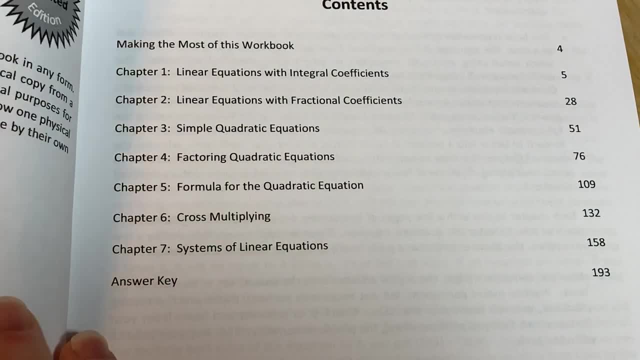 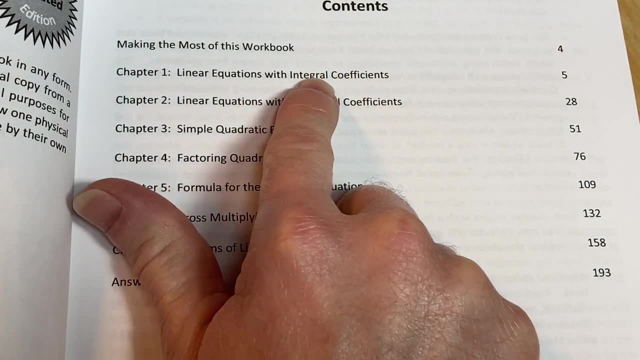 just show you some of the topics And it's very limited in the topics. but what it does have it covers well. So linear equations with integral coefficients. that basically means the coefficients are whole numbers, so like: 2x plus 5 equals 0.. Linear equations. 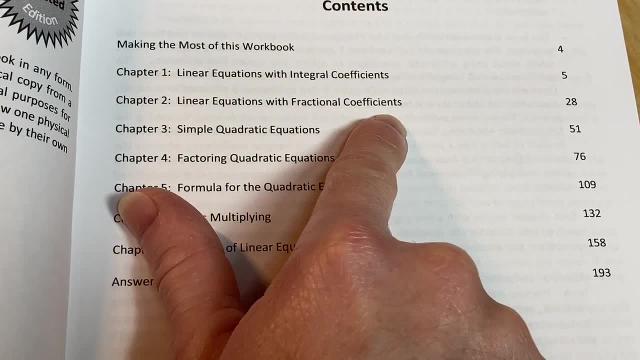 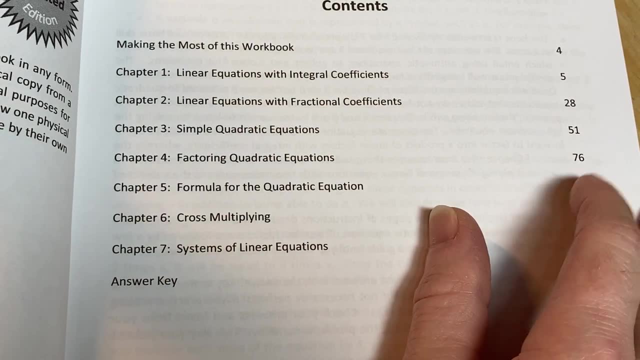 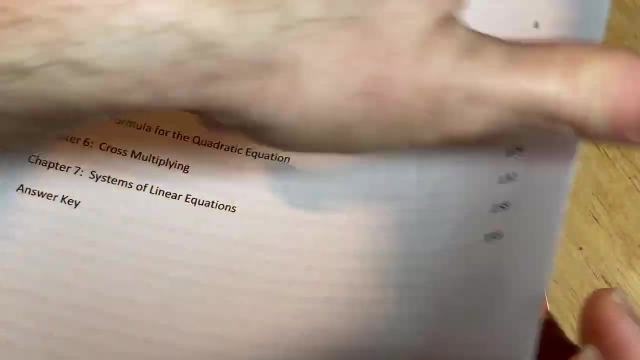 with fractional coefficients. that basically means you have fractions in the equation, Simple quadratic equations, factoring quadratic equations, formula for the quadratic equation, cross-multiplying and systems of linear equations, So very, very restricted in terms of its topics and it has an answer key, so you have answers to every single problem. 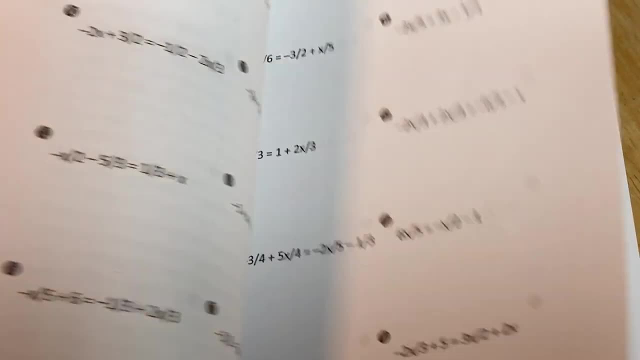 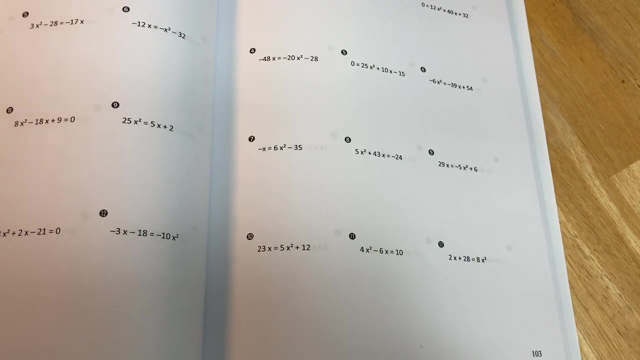 So again, both of these books are really, really for beginners. I want to emphasize that because they don't have everything, They're not textbooks, but what they do cover, they cover well. So again, both of these books are really, really for beginners. I want to emphasize 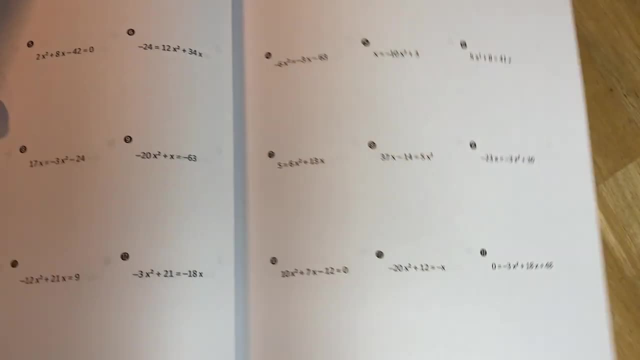 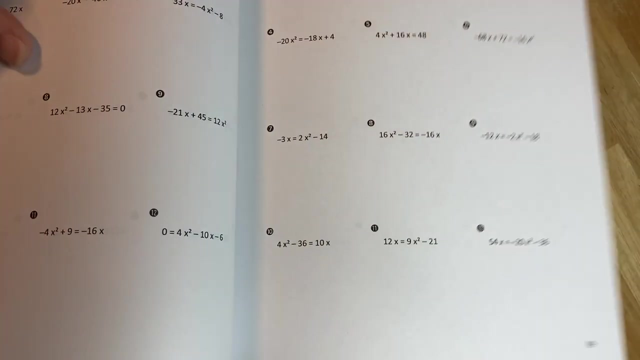 that. So you have tons of problems. I mean, look at all of these quadratic equations. I mean this is crazy, right? There's so many problems here, It's insane. It's just problem after problem after problem and you see that you can write in the book, which I think makes. 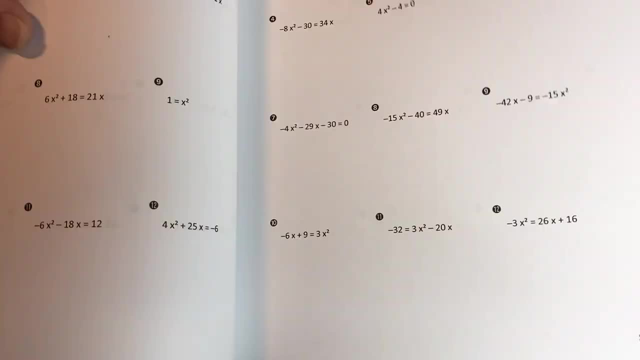 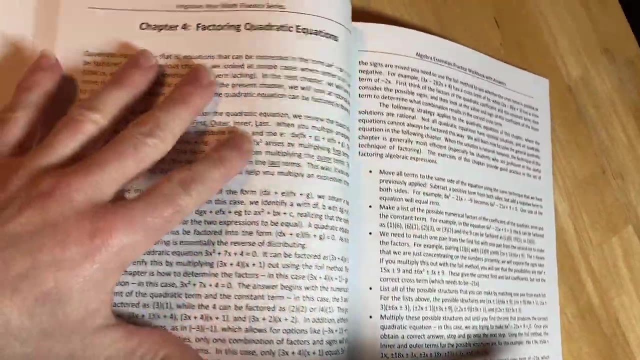 them a really good choice for people who are learning. I mean, look at this, It's just insane how many problems there are in this book. So how the books work, are you have, like a little introduction? The author, Chris McMullen. 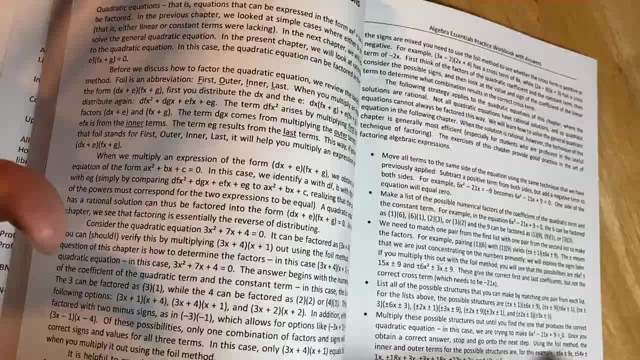 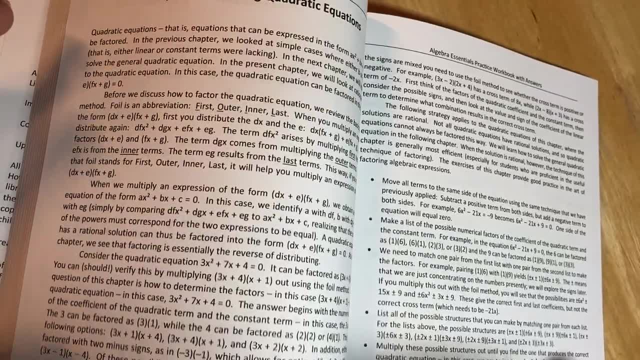 does a really good job, job trying to explain everything. I feel like the explanations in this book- the examples, the verbal explanations- are very similar to what you would get from watching like a YouTube video, So he takes extra effort in explaining. It doesn't really read like a regular textbook. So if you've 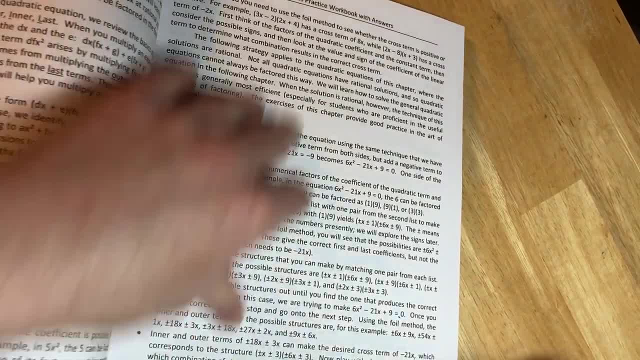 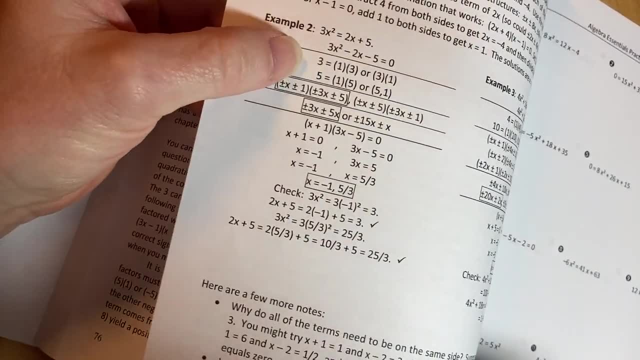 tried regular math books. this might be something to try. And then, after you go through everything, he gives you some examples, as you can see here. I mean he just goes into painstaking labor here to explain how to factor. I mean he shows you all the possibilities and then how to check your. 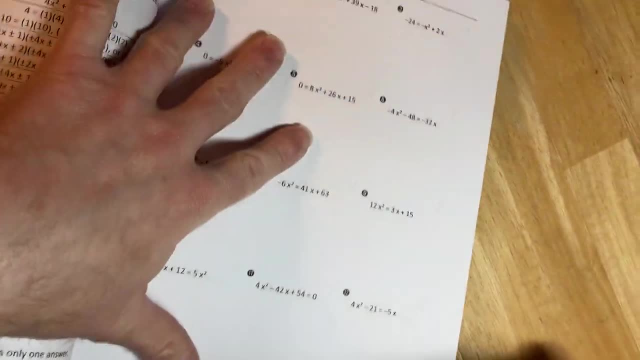 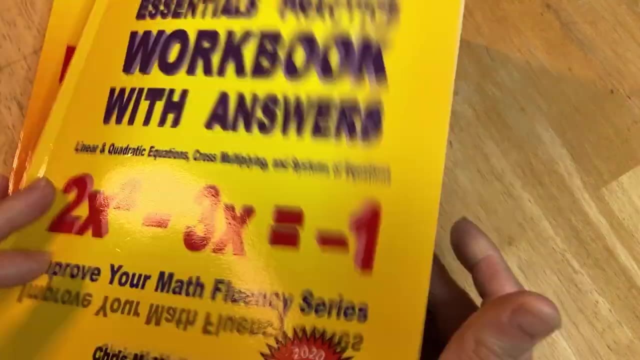 answer and then how to solve the equation. And then here you can see you have the examples, And then you can look in the back of the book and just check your work. So how do you use books like these? Like, let's say, you buy one of these books. I'll leave links in the description so you can. 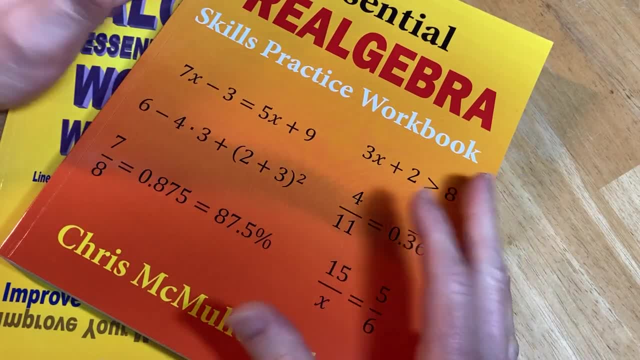 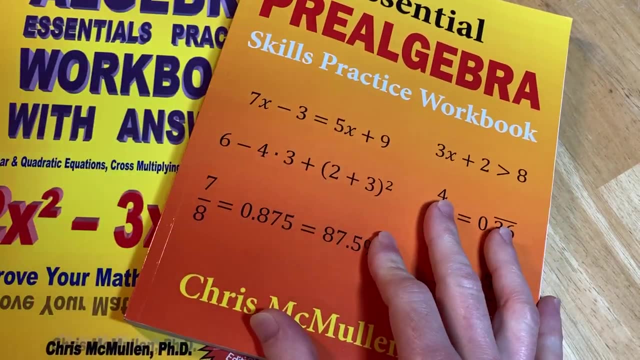 check them out. Let's say you buy one. What do you do, right? So my advice is to try to do at least one problem every day, Like if you can get yourself to sit down and do one problem from whichever one. 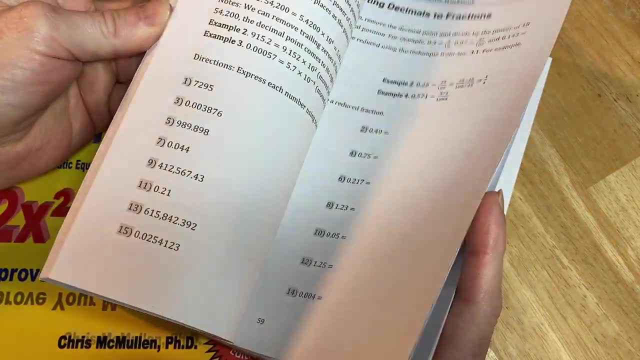 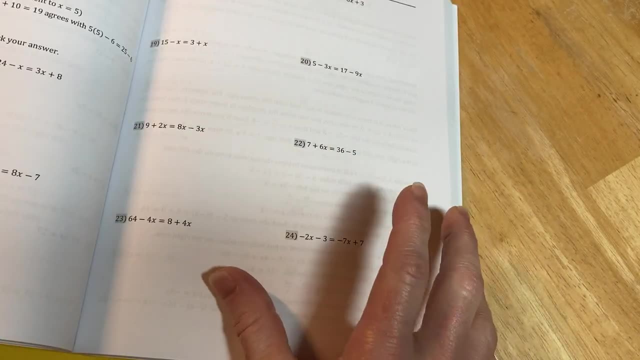 I think you're going to get better at math And you might say, well, is one problem really enough? Well, you could tell yourself that you're going to do an hour of mathematics every day, But what I have found with most people who do that is that they can't keep it up, And it's not. 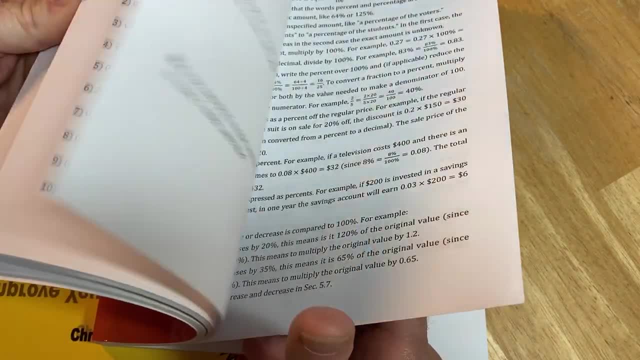 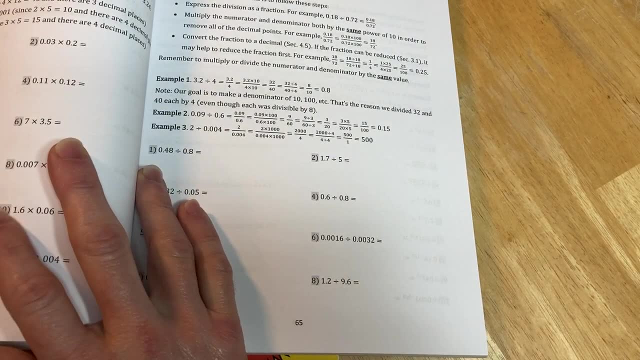 because they're not disciplined or because they're lazy. It's just because, as human beings, when we see a task in front of us and it's like an hour a day, on some days we're not going to want to do it, because some days we're going to be distracted right, Some days you're going to have, you know. 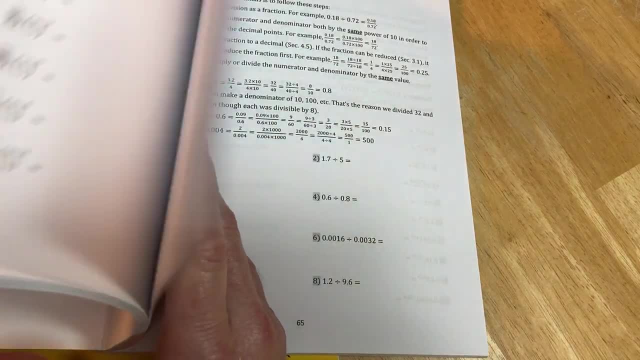 problems, right, And then you're going to have to do it, And then you're going to have to do it. You might be sick, You might have a problem with your friend or your significant other, You might have a problem at work, You might have other responsibilities. So if you tell yourself you're, 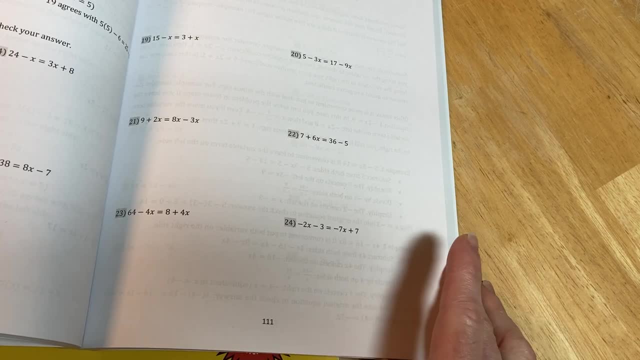 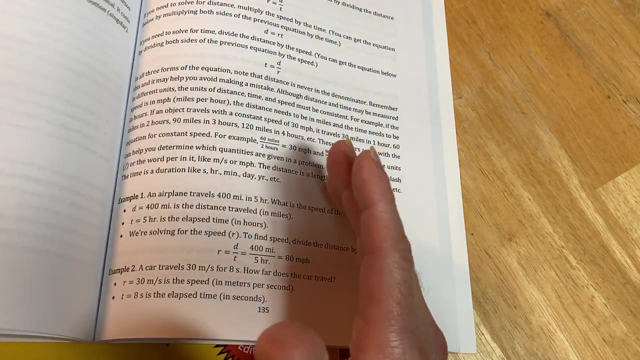 going to do at least one math problem a day. I think it's just a good way to get yourself to do it. And once you sit down, once you get a piece of paper and you sit down and, like you start doing a problem from one of these books, you're in the zone. You know what I mean. You're thinking And 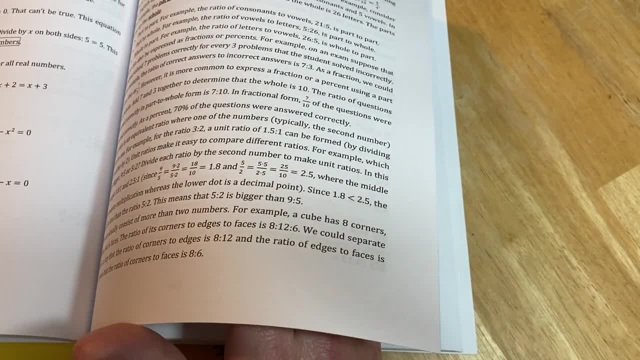 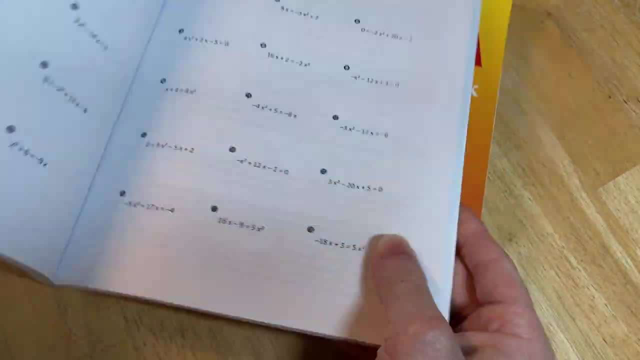 if you do it in the morning. I think the morning is the best time. This is just for me. You'll think about it the rest of the day. You know, if you solve a quadratic equation from this book in the morning and then you go to work or you go to class or whatever, you'll be like: oh yeah, what did? 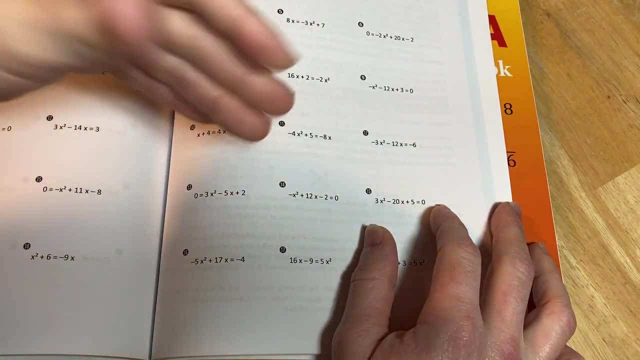 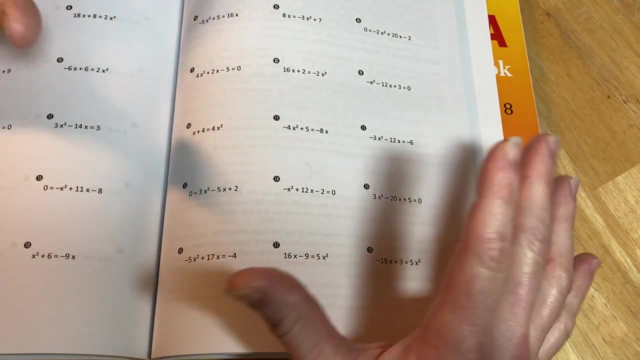 you do this morning. Well, you solved the quadratic equation. You've already done something good for your day. You've already like, owned the day. You've done something productive, You've moved forward in your life somehow, because you've learned some mathematics for that day And the 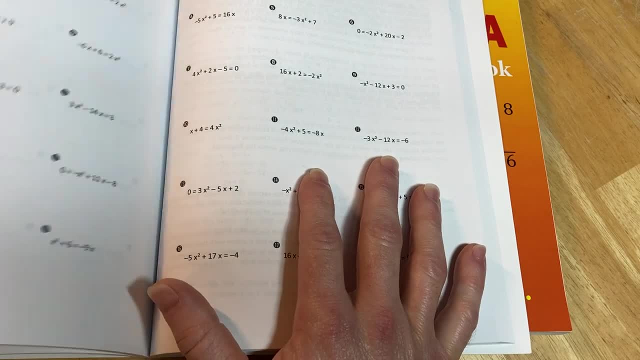 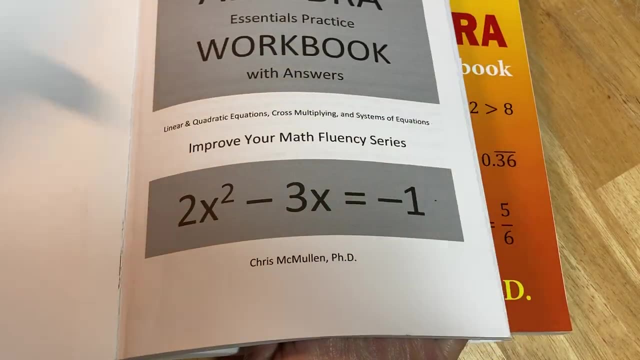 rest of your day is just whatever. You know you've accomplished something And I think that says something about you know doing math every day. You know it's like training your mind every day. Now, these books aren't perfect. Again, they're workbooks. They don't have 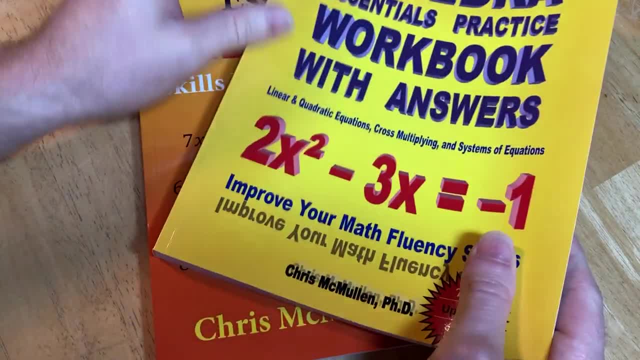 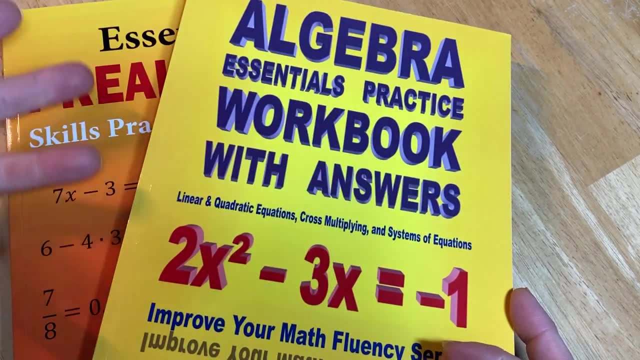 everything, But they're super affordable. You can write in them And they will make you better at mathematics, right, They'll make you better at math, And if you actually did every problem in these books, I mean you would know everything. in these books There's just so much, so many. 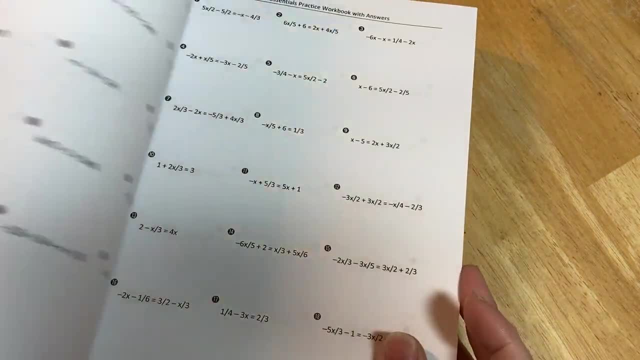 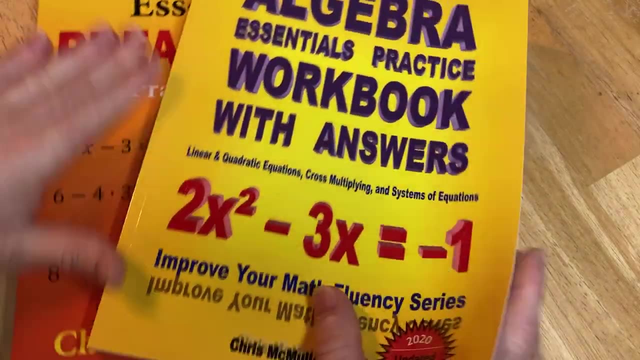 practice problems that I don't think it's realistic for someone to sit down and do them all, But that's good right, Because you'll always have enough problems to do, which is really good. So again, this one is for For super, super beginners, pre-algebra, if you just like, don't know much at all, I mean. 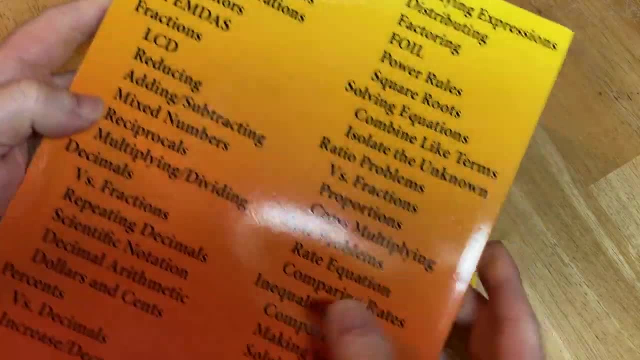 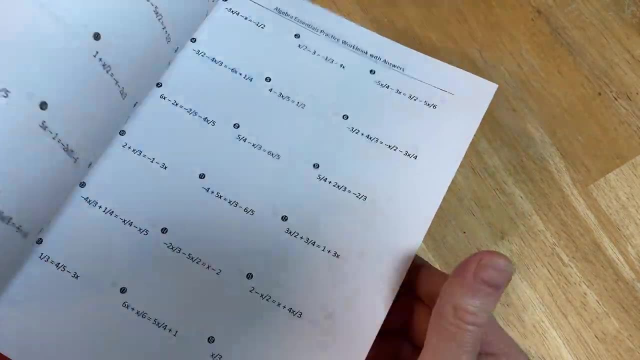 it's just. Here's some of the topics in the back: Really basic stuff, right Adding, subtracting fractions, decimals, stuff like that. And then here this is for someone who's going into actual algebra- It's called algebra, whereas this one is pre-algebra. So, And again, not perfect. 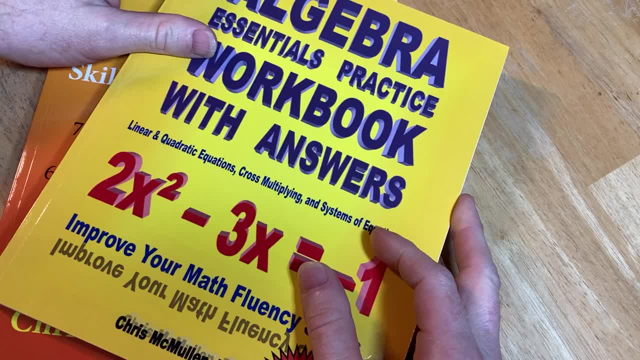 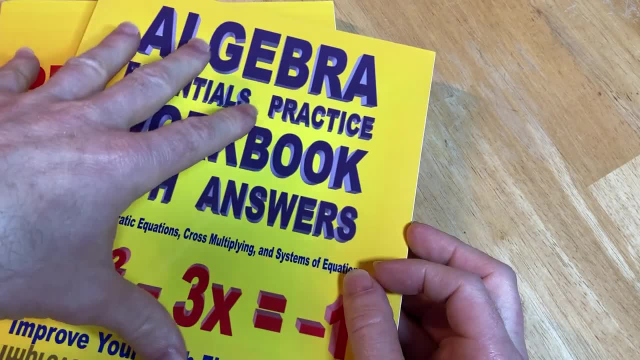 but super awesome. I'll leave links in the description in case you want to check these out. I also have math courses, But my math courses actually start at the level, At the algebra level. So My courses, My college algebra course, has everything in this book and like way more.